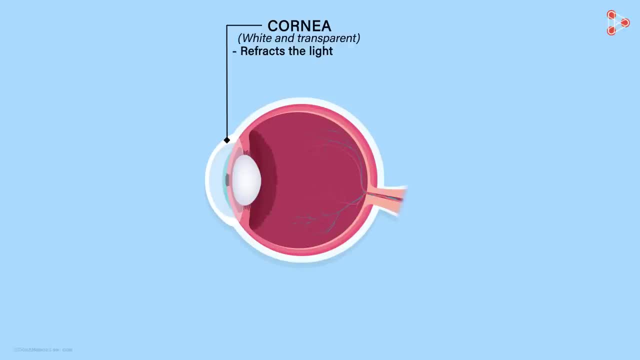 It not only refracts light but also protects the inner parts of the eye. It acts like a tough front wall of the eye, protecting the interior of the eye from accidents, and also does not allow foreign particles to enter. Okay, So this was all about the outer layer of the eye. 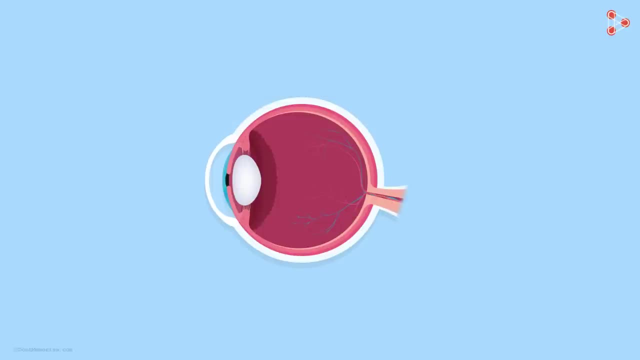 Let's now talk about the things present inside. Behind the cornea, there is a dark muscular structure called the iris. Iris determines the colour of the eye. For instance, when we say that a person has blue eyes, it means that the colour of the 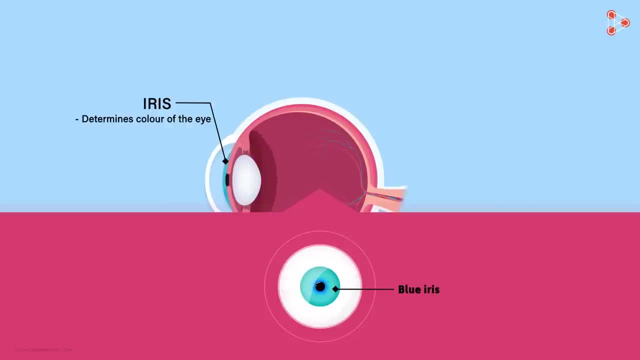 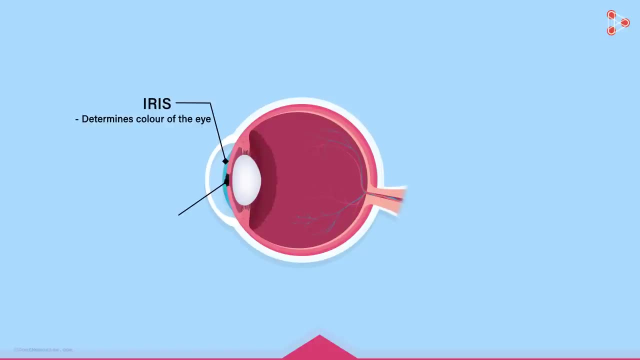 iris of the person's eye is blue. Now there is a small opening at the centre of the iris for the light to enter. Do you know what it's called? It's called the pupil. The iris actually acts like a shutter of a camera. 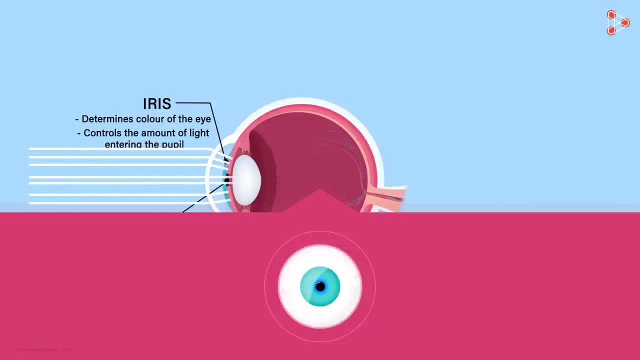 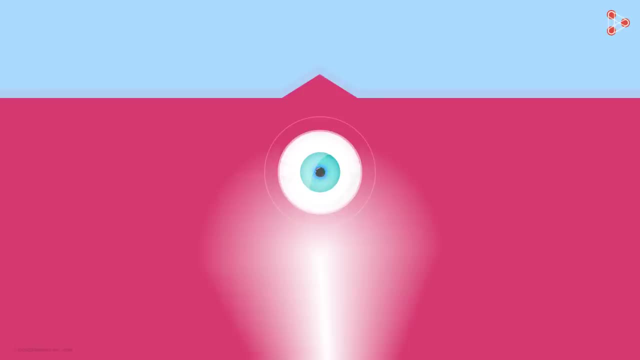 It controls the amount of light entering the eye by enlarging or shrinking and thereby adjusting the size of the pupil. For example, when you focus the light from the top of the pupil, it controls the amount of light entering the pupil. When you focus the light from the torch directly into a person's eye, the iris shrinks. 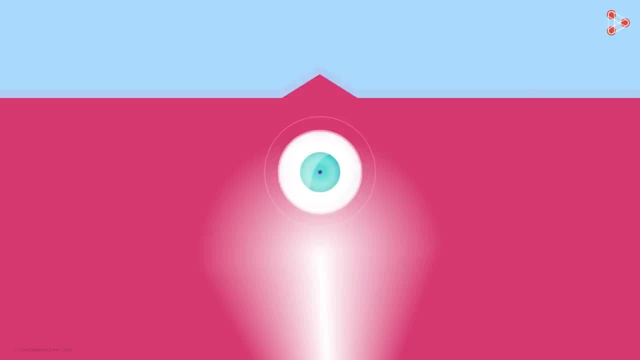 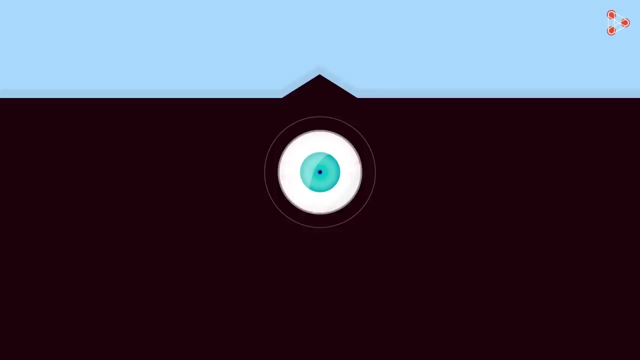 This is because the intensity of light is too much for the eyes to bear. The shrinking iris stops the unwanted light from entering through the pupil, And when there is less light, it expands, allowing more light to enter through the pupil. Okay, What happens next? 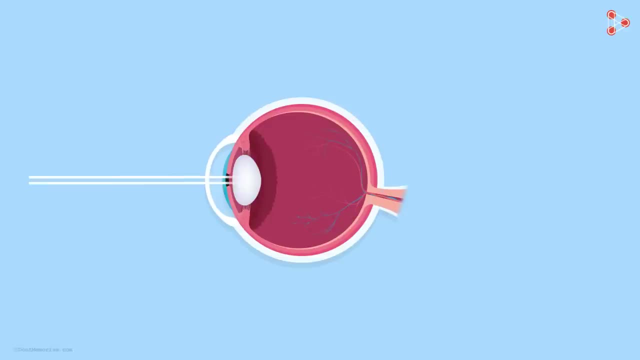 The light that enters through the pupil falls on the lens kept behind The lens is a convex lens. Convex lens is a lens which is thicker at the centre than the edges. It's a converging lens, That is, it focuses all the light at one point. 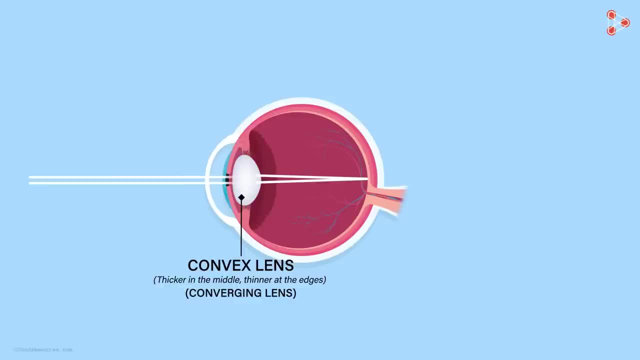 In a normal, regular eye, this point is somewhere here, on this inner boundary called retina. Why do I say a normal eye? Well, in a defective eye, this point of focus may lie either in front of the retina or behind the retina. 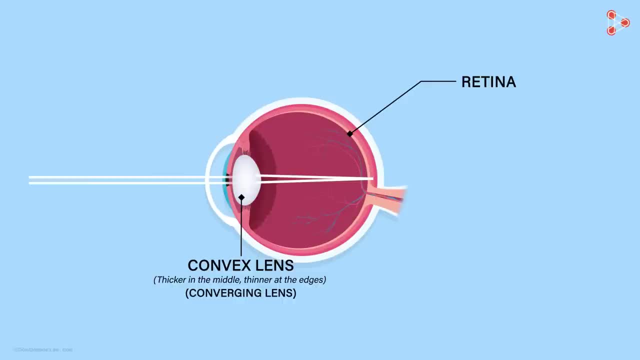 We will talk about this defect of eye in our future videos, But first let's go back to our normal eye, where light is focused on the retina. Retina is at the back of the eye and marks the inner layer of the eyeball.